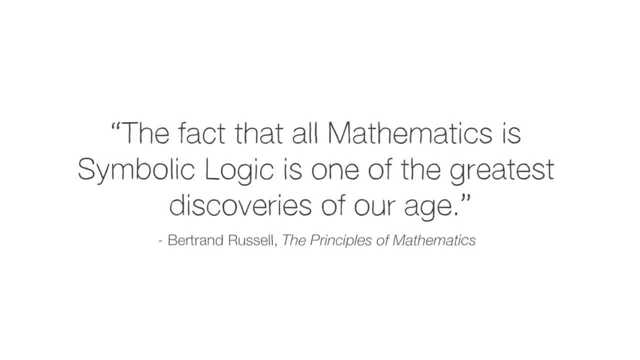 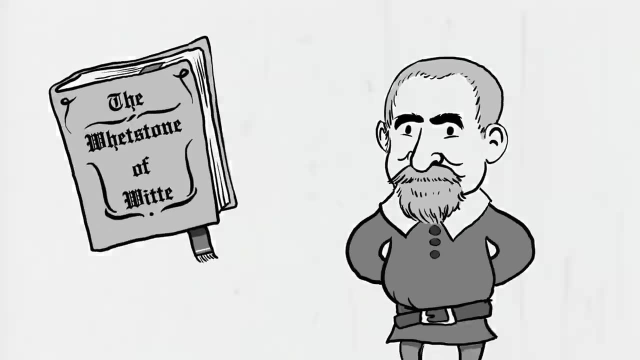 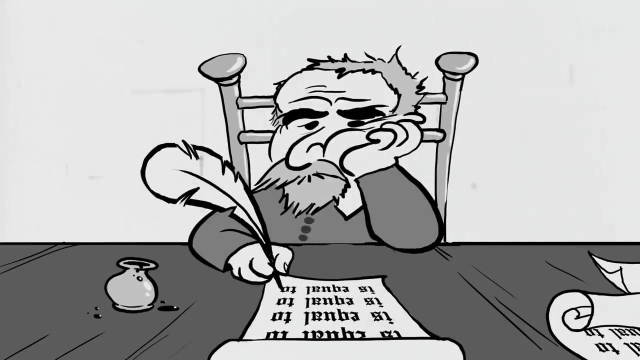 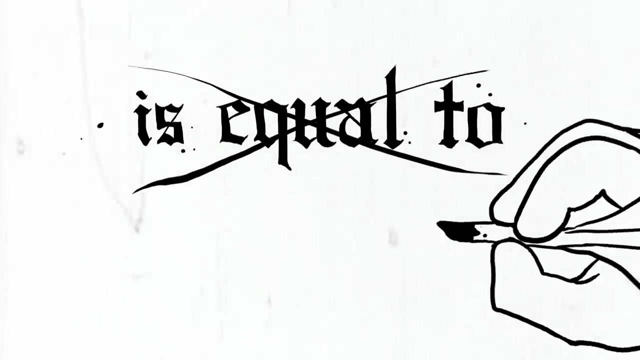 In the 16th century the mathematician Robert Record wrote a book called The Whetstone of Wit to teach English students algebra. But he was getting tired of writing. the words is equal to over and over. His solution: He replaced those words with two parallel horizontal line segments. 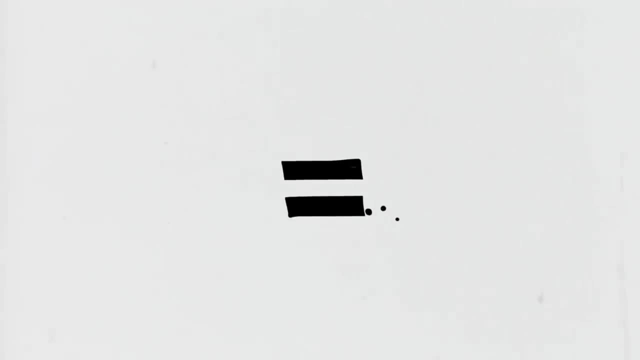 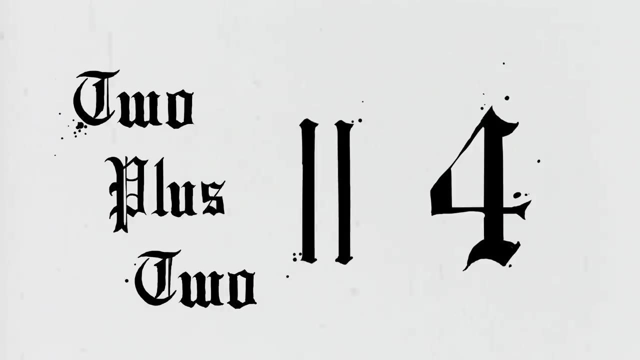 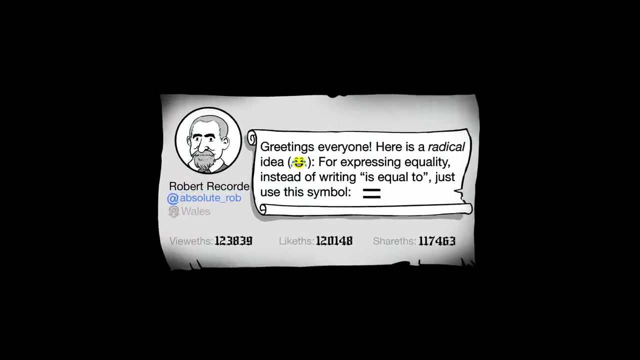 because, the way he saw it, no two things can be more equal. Could he have used four line segments instead of two? Of course, Could he have used vertical line segments? In fact, some people did. There's no reason why the equal sign had to look the way it does today. 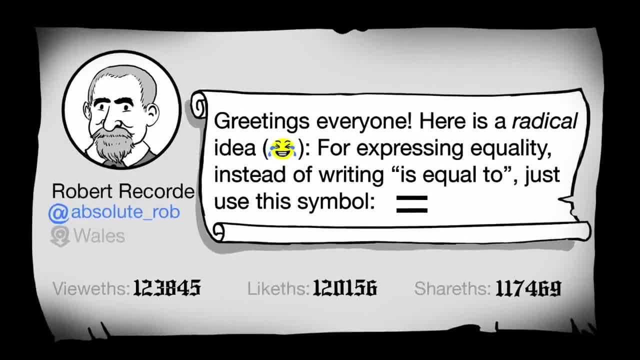 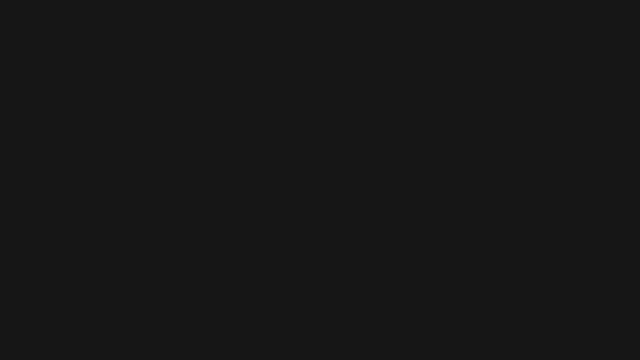 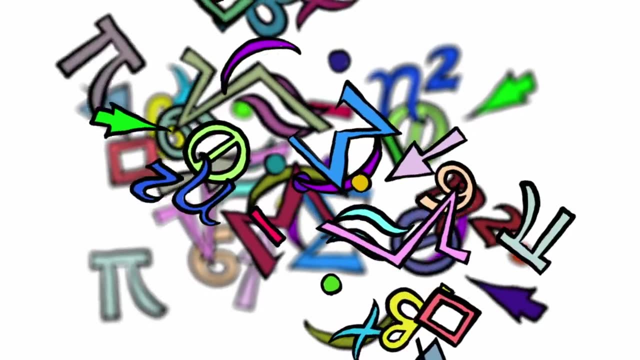 At some point it just caught on sort of like a meme. More and more mathematicians began to use it and eventually it became a standard symbol for equality. Math is full of symbols: Lines, dots, arrows. English letters, Greek letters, superscripts, subscripts. 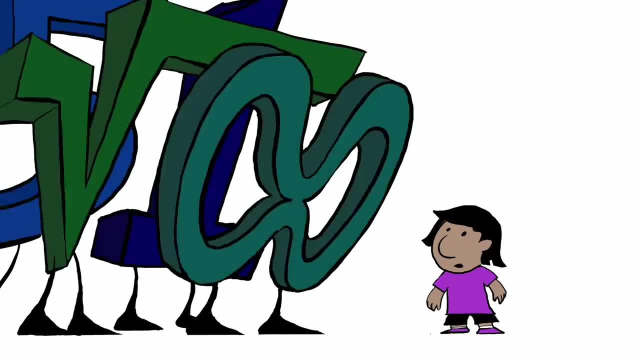 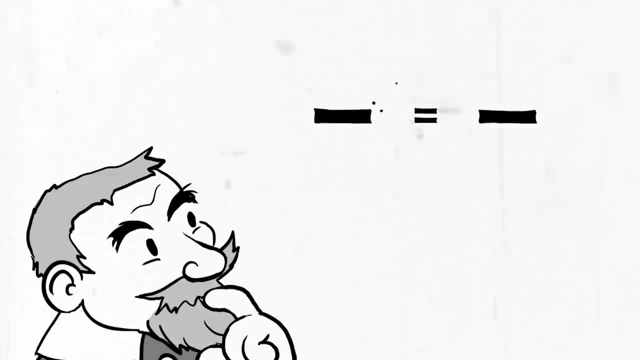 It can look like an illegible jumble. It's normal to find this wealth of symbols a little intimidating and to wonder where they all came from. Sometimes, as Record himself noted about his equal sign, there's an apt conformity between the symbol and what it represents. 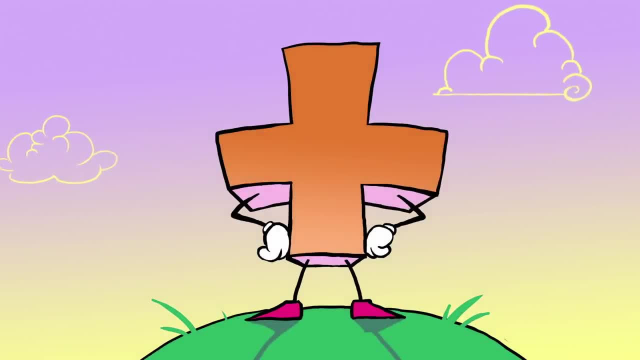 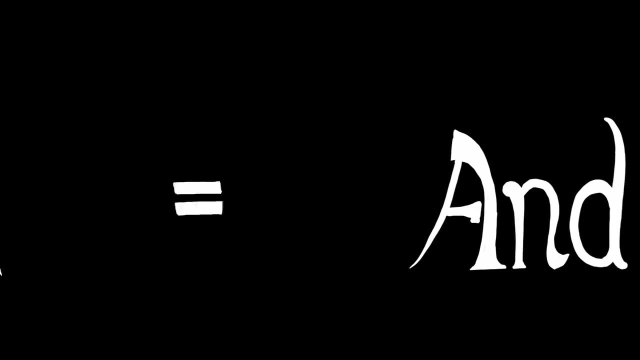 Another example of that is the plus sign for addition, which originated from a condensate. It's the guessing of the Latin word et, meaning, and Sometimes, however, the choice of symbol is more arbitrary, such as when a mathematician named Christian Cramp. 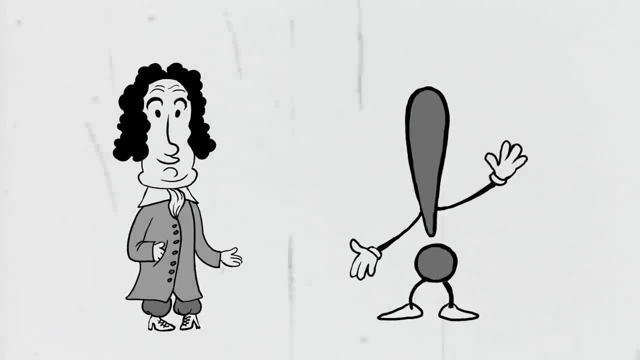 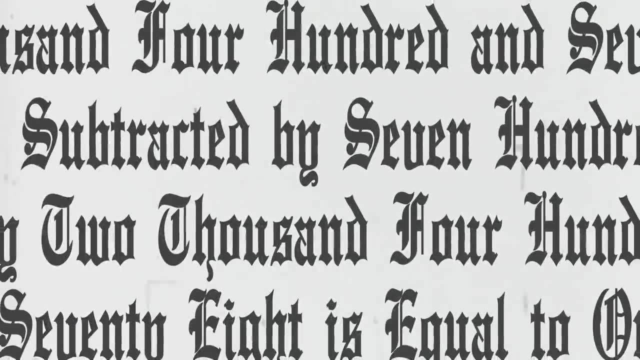 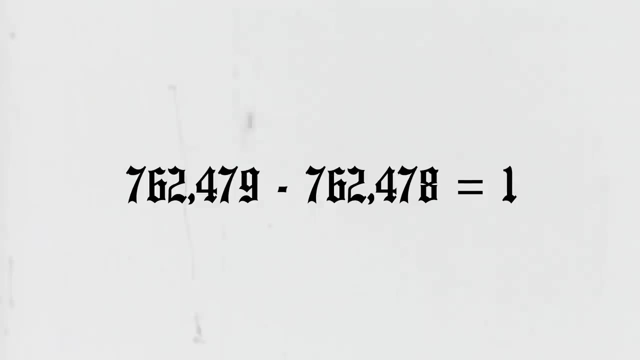 introduced the exclamation mark for factorials just because he needed a shorthand for expressions like this. In fact, all of these symbols were invented or adopted by mathematicians who wanted to avoid repeating themselves or having to use a lot of words to write out mathematical ideas. 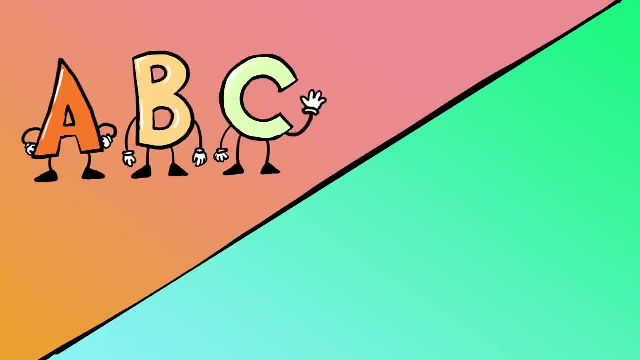 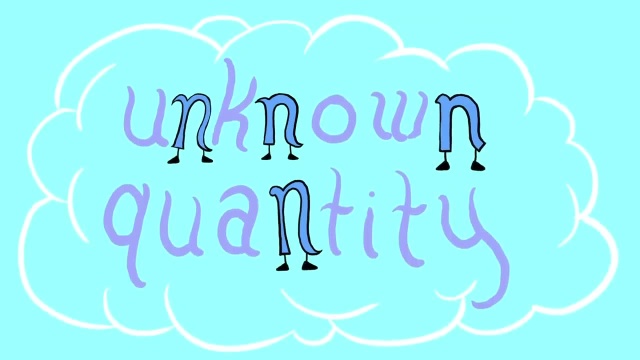 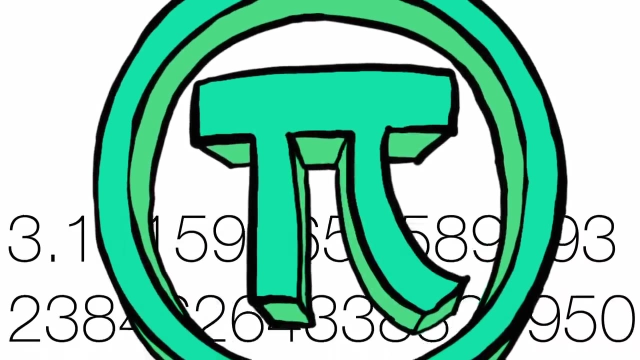 Many of the symbols used in mathematics are letters, usually from the Latin alphabet, or Greek Characters are often found representing quantities that are unknown and the relationships between variables. They also stand in for specific numbers that show up frequently but would be cumbersome or impossible to fully write out in decimal form. 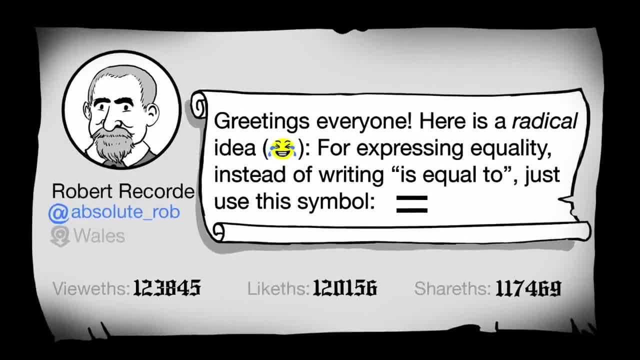 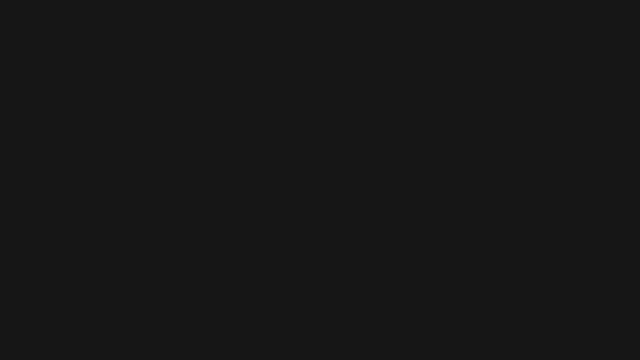 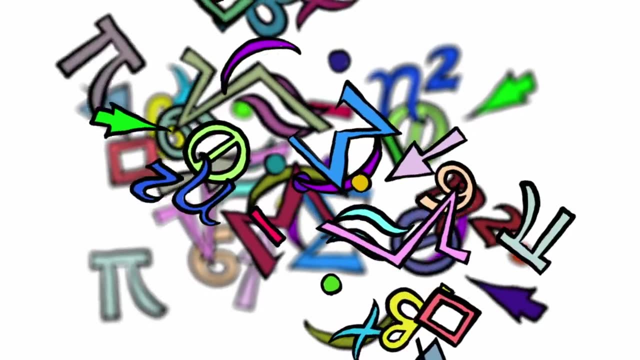 At some point it just caught on sort of like a meme. More and more mathematicians began to use it and eventually it became a standard symbol for equality. Math is full of symbols: Lines, dots, arrows. English letters, Greek letters, superscripts, subscripts. 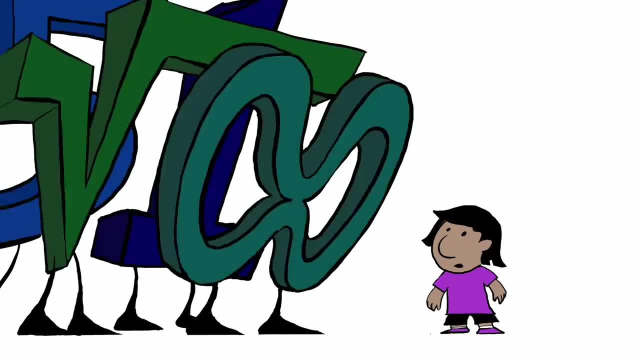 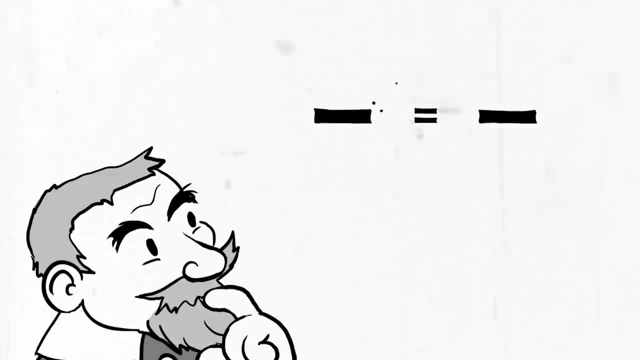 It can look like an illegible jumble. It's normal to find this wealth of symbols a little intimidating and to wonder where they all came from. Sometimes, as Record himself noted about his equal sign, there's an apt conformity between the symbol and what it represents. 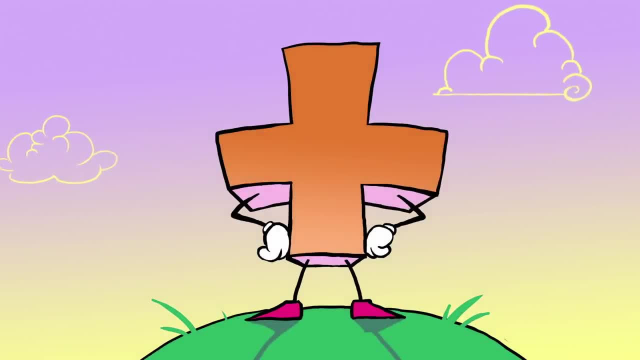 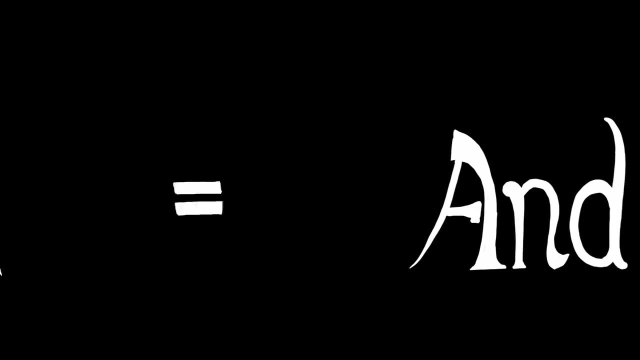 Another example of that is the plus sign for addition, which originated from a condensate. It's the guessing of the Latin word et, meaning, and Sometimes, however, the choice of symbol is more arbitrary, such as when a mathematician named Christian Cramp. 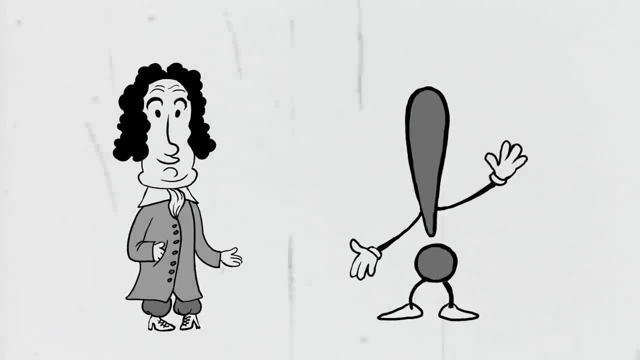 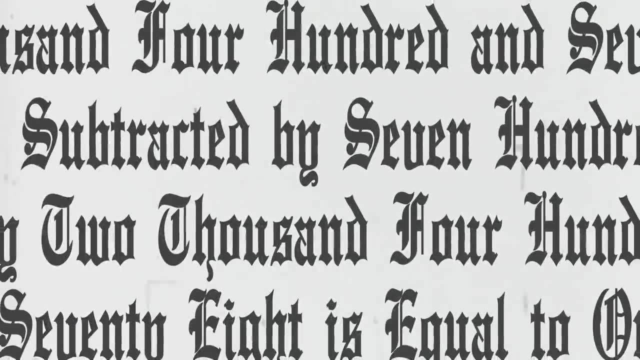 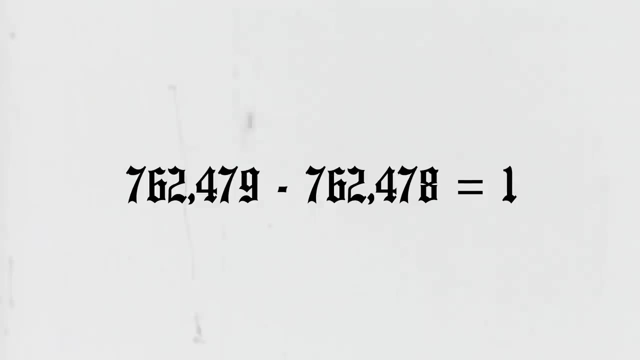 introduced the exclamation mark for factorials just because he needed a shorthand for expressions like this. In fact, all of these symbols were invented or adopted by mathematicians who wanted to avoid repeating themselves or having to use a lot of words to write out mathematical ideas. 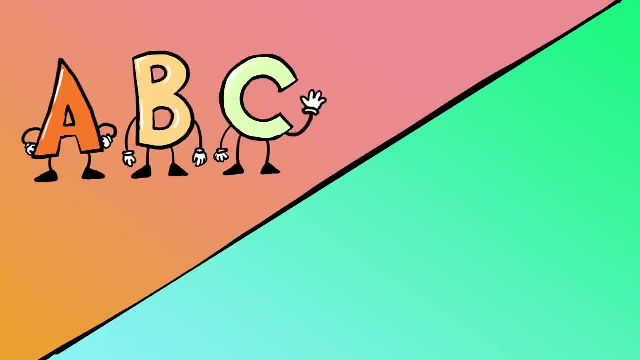 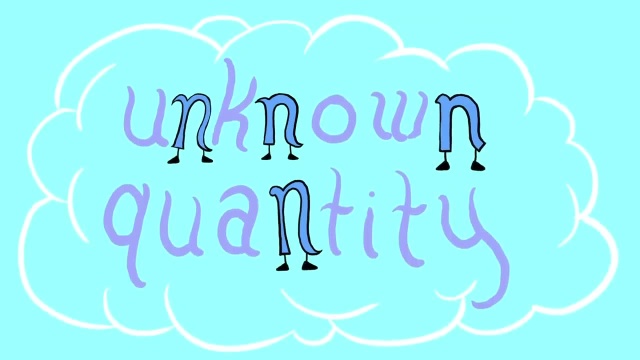 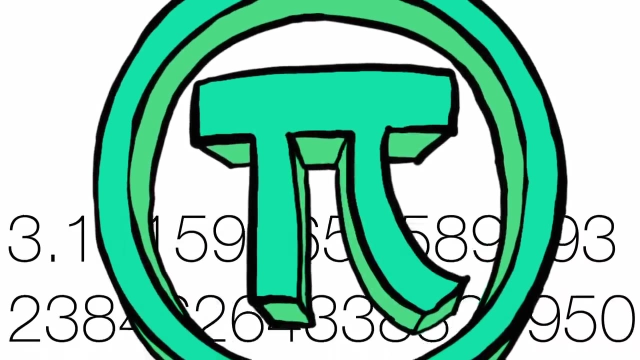 Many of the symbols used in mathematics are letters, usually from the Latin alphabet, or Greek Characters are often found representing quantities that are unknown and the relationships between variables. They also stand in for specific numbers that show up frequently but would be cumbersome or impossible to fully write out in decimal form. 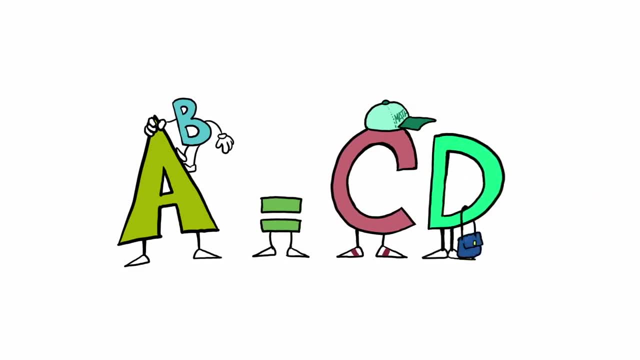 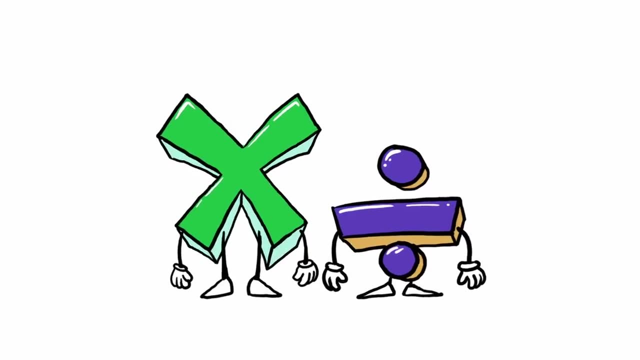 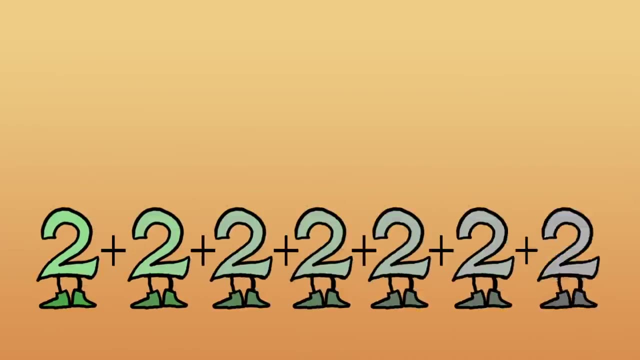 Sets of numbers and whole equations can be represented with letters too. Symbols are used to represent operations. Some of these are especially valuable as shorthand, because they condense repeated operations into a single expression. The repeated addition of the same number is abbreviated with a multiplication sign. 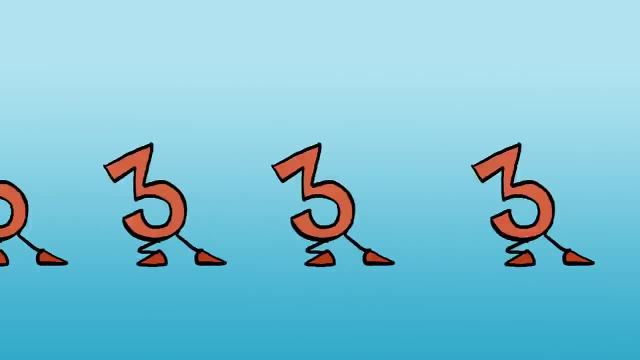 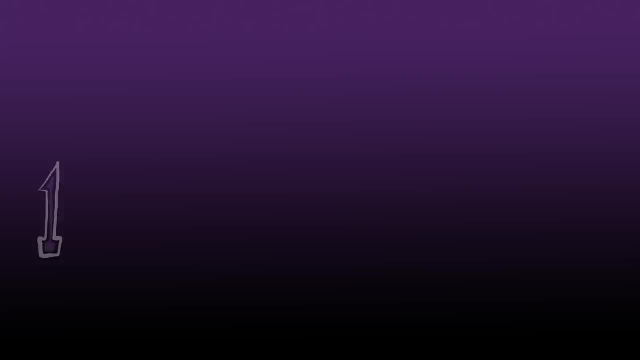 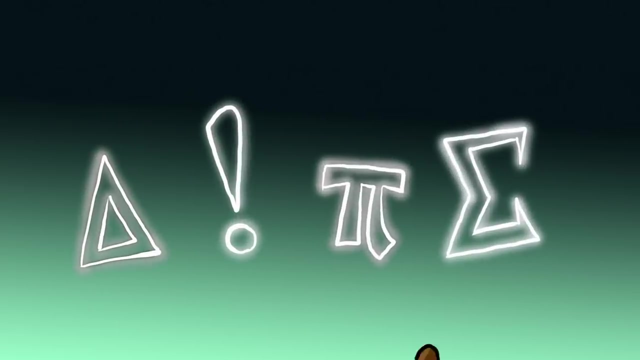 so it doesn't take up more space than it has to. A number multiplied by itself is indicated with an exponent that tells you how many times to repeat the operation, And a long string of sequential terms added together is collapsed into a capital sigma, which means that the number of times to repeat the operation is smaller than the number of times to repeat the operation.